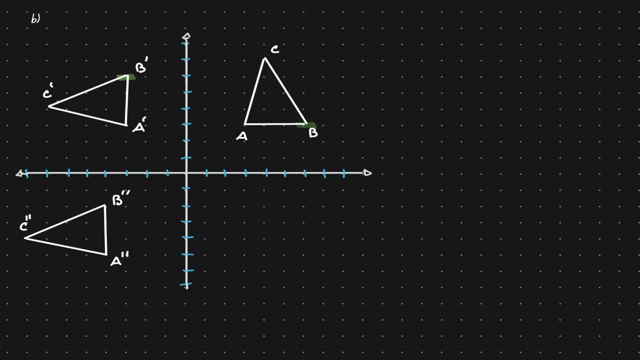 it's in the top, So a reflection, it's out of the question as well. So how about we think about rotation? Because notice that it kind of seems like a reflection. but it's actually a reflection. It seems like there was a rotation C. if we kind of rotate it counterclockwise, it kind of lands. 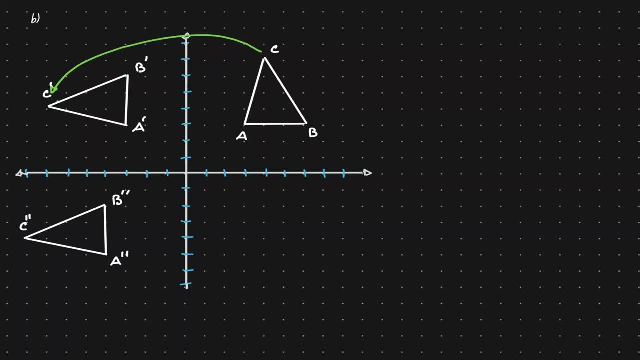 at this position, And B if we kind of rotate it counterclockwise, it kind of lands at this position, And A if we rotate it counterclockwise. So this is a clear indicator that there was some kind of rotation involved. But we need to be specific, We need to indicate how many degrees. 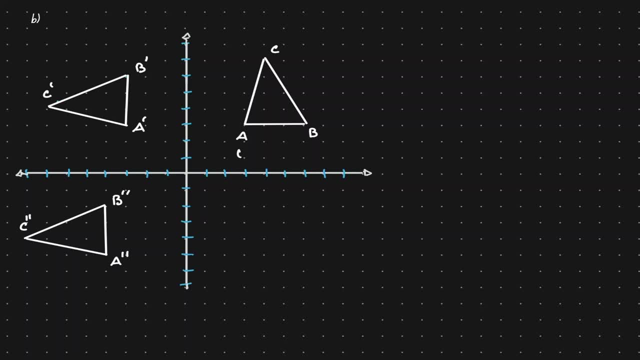 that we rotated. Let's look at the coordinate points. So if we concentrate at point B, notice that the coordinate point 6 comma 3, it became negative 3 comma 6. So they kind of switch position and then we change the x value And that also goes. 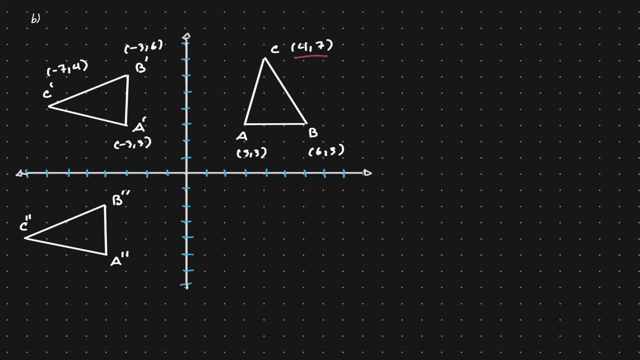 for coordinate point C It was 4 comma 7, and then it became negative, 7 comma 4.. So it's the same behavior. So if we concentrate at point B, notice that the coordinate point 6 comma 3, it became 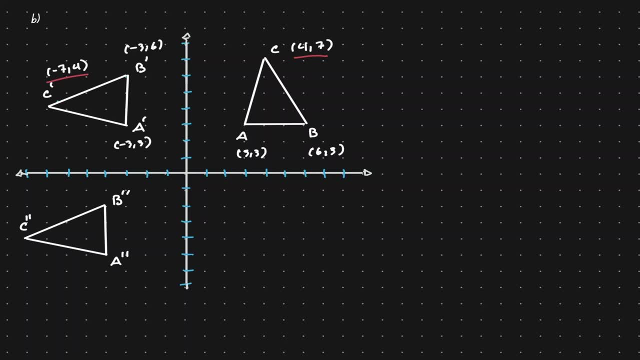 negative. 7, comma 4.. So it's the same behavior. We switch locations and then we change the new value of x And notice that that is the rule When we rotate 90 degrees, when the center of rotation it's at. 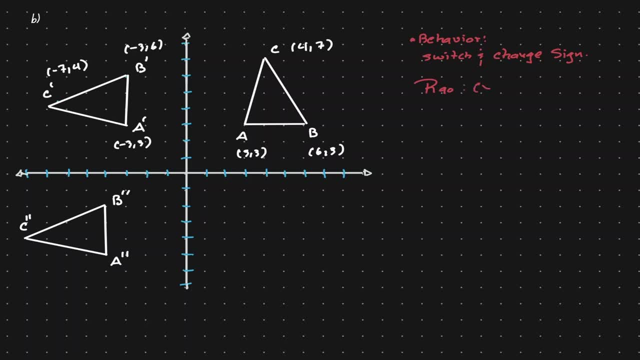 the origin, Any coordinate point: x comma y. the image is negative: y comma x. So we have identified the first transformation. It is a transformation. It is a transformation of a rotation of 90 degrees. So now let's think about what needs to happen for the upper left triangle to land exactly on the. 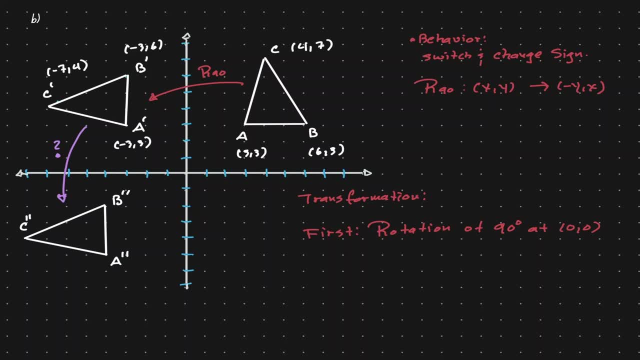 bottom triangle for us to identify the second transformation. If we take a look into terms of orientations, we'll see that the first transformation is a rotation of 90 degrees And the second transformation is a rotation of 80 degrees. Notice that A prime